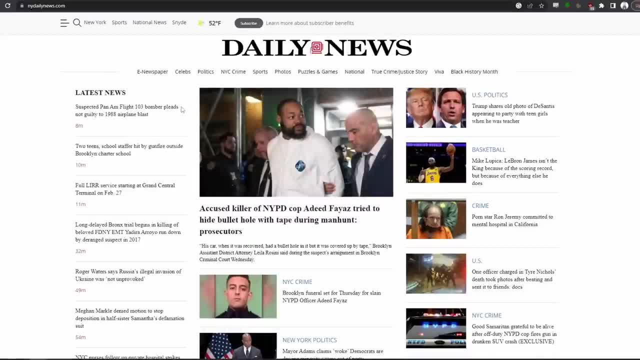 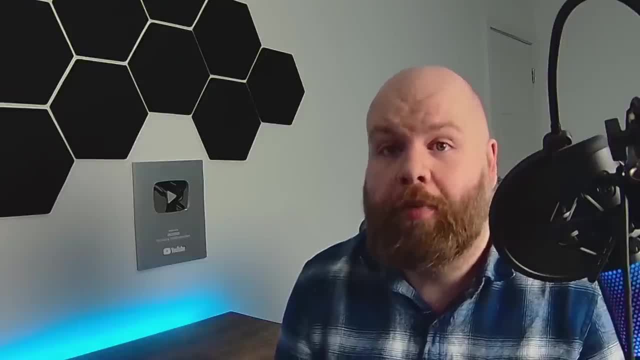 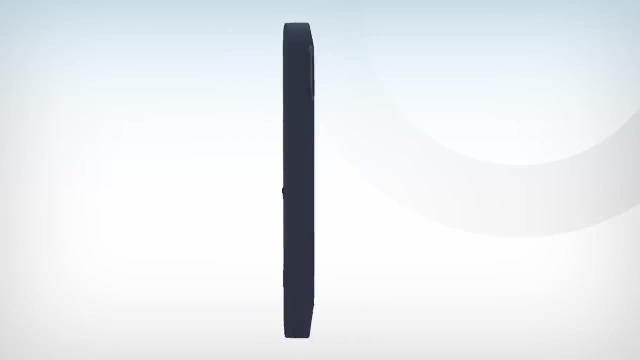 Private Internet Access is the world's most transparent VPN service. They keep no user logs and it has 100% open source, publicly available source code. PIA even had their entire network and management systems independently audited to demonstrate that they keep no logs. 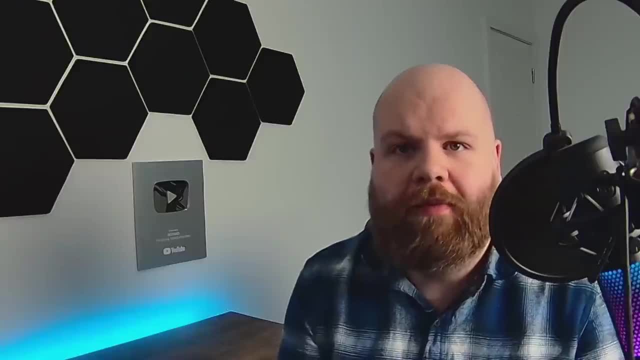 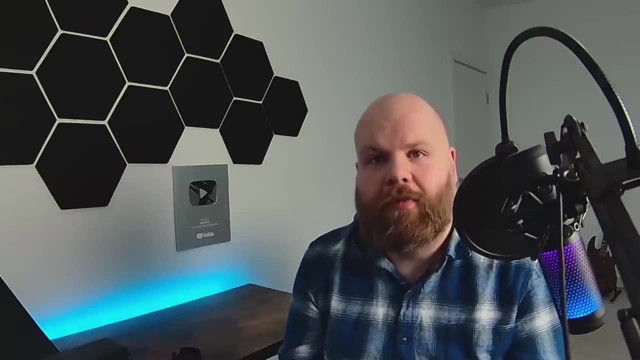 Private Internet Access works with all major streaming services and websites, and it's one of the few VPNs that actually allows you to access peer-to-peer file sharing. By clicking on the link in the description box, you'll get an 83% discount on Private. 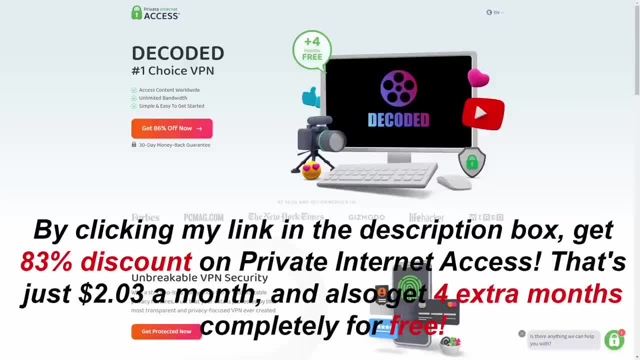 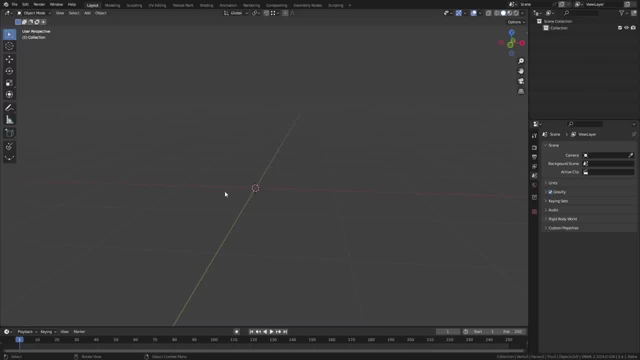 Internet Access. That works out to just $2.03 a month, and you'll also get an extra four months completely for free. So let's jump into Blender and take a look at some of these topology tips. Tip number one is about controlling hard surface details on curved surfaces. Often, if you'll 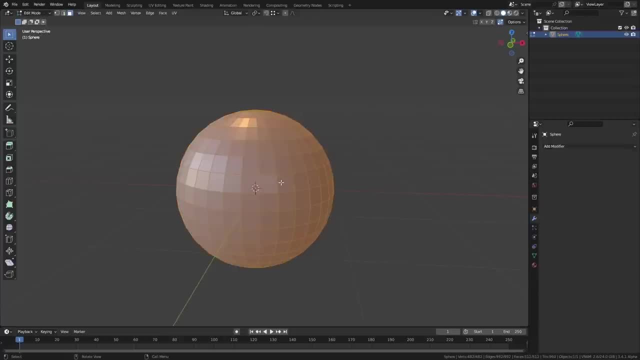 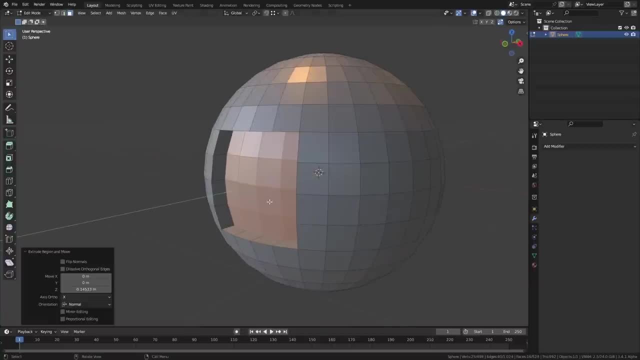 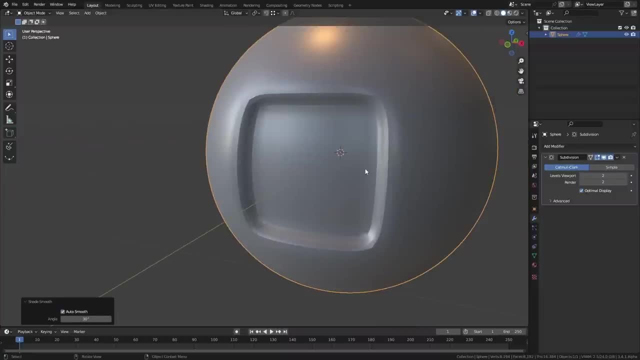 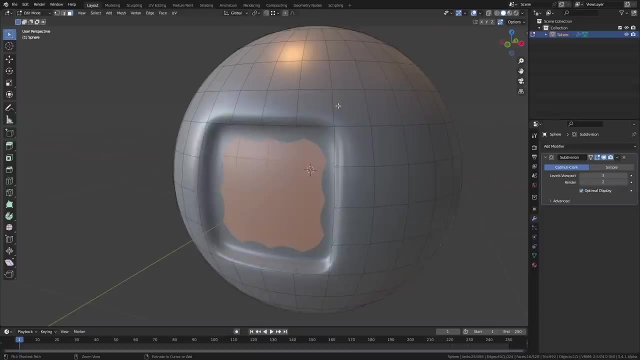 modifier and it all goes a little bit too curved. So you think to yourself: oh well, what I'll do is I'll add some supporting loops, right, Because if you put a loop next to another edge, it'll tighten that surface up. So you add in these loops and you bring it in like 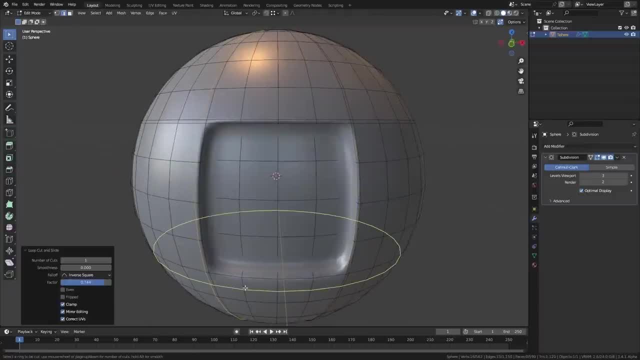 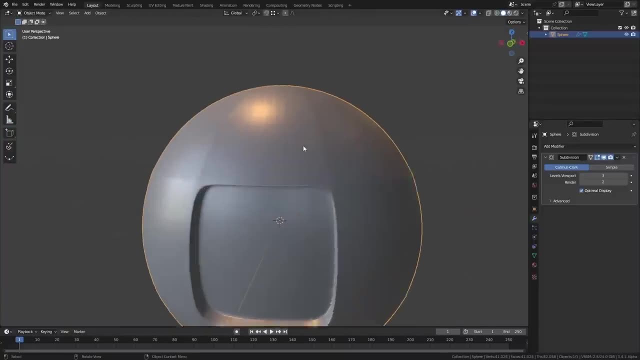 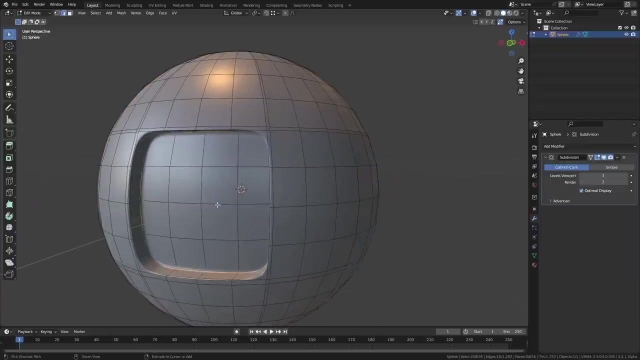 this and like this and like that and maybe you put one around here And you think that looks pretty good. You go into object view and you see that you have these horrible crease marks. We can fix that really easily. There's two main ways of doing that, but you don't want to use supporting. 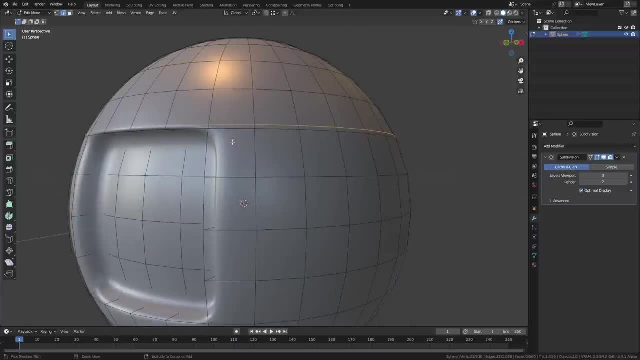 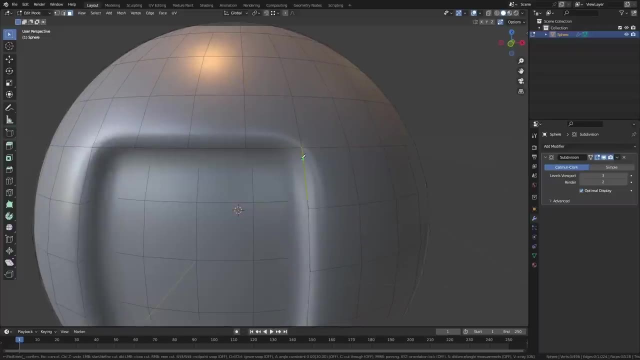 edges that go all the way around like this, because it will just cause pinching and it'll cause problems. So the first way that you can do this, if you really want to use supporting edges, what I would suggest you do instead is use the knife tool. find a nearby vert. 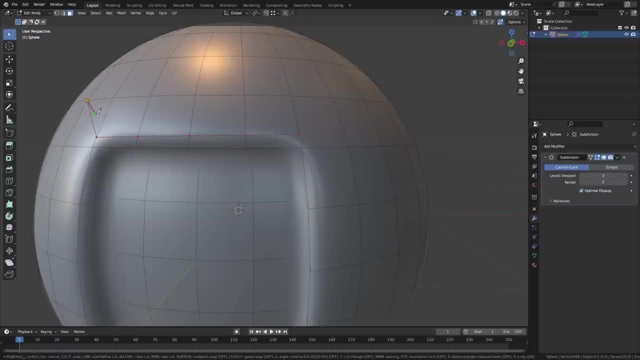 bring it across something like this and just manually cut in onto the surface, And if we look at this in object mode, we have none of that weird pinching that we had before, but we still get the nice hard line. The other thing that you can do- and this is probably 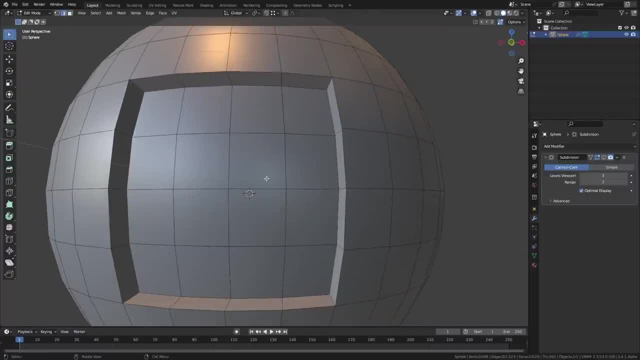 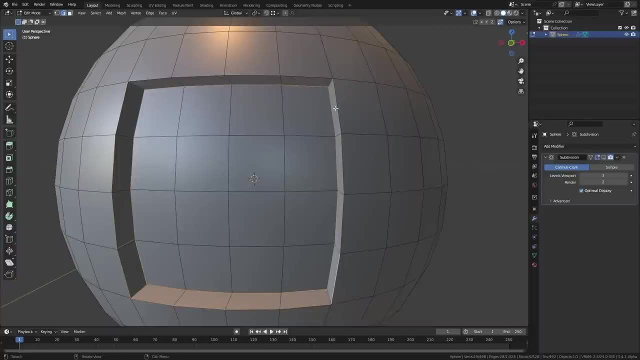 my preferred method if I'm working on something like this is to select around the edges and use creasing instead. Subdivision surface modifiers basically work by adding new faces in between the original faces that are there, and then it averages out the position of all. 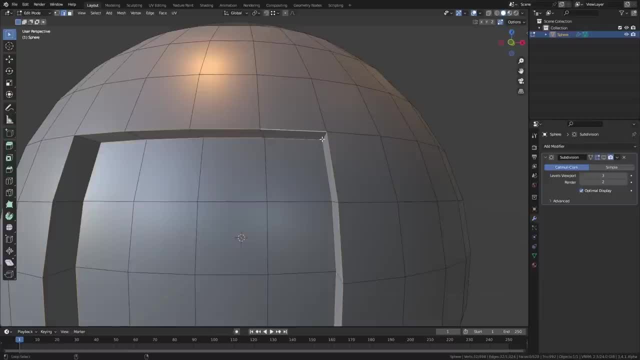 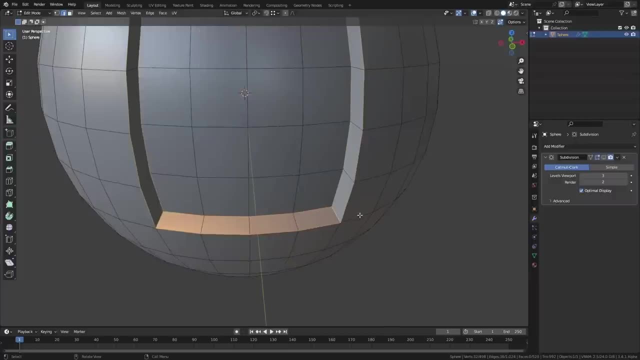 the faces based on the closest neighbors. So when you use creasing, you're basically all that you really do. is you change how much that's going to get averaged out by? So if we select all of these and we use shift and E to add crease, you can see that the 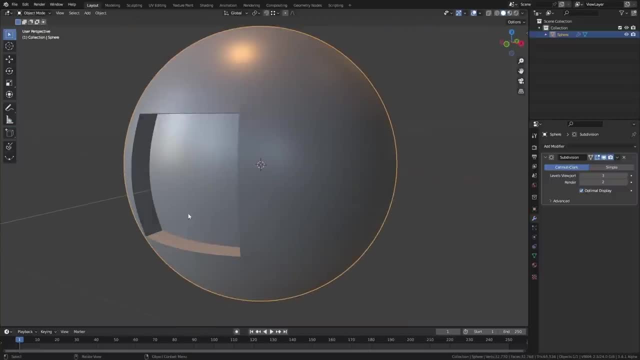 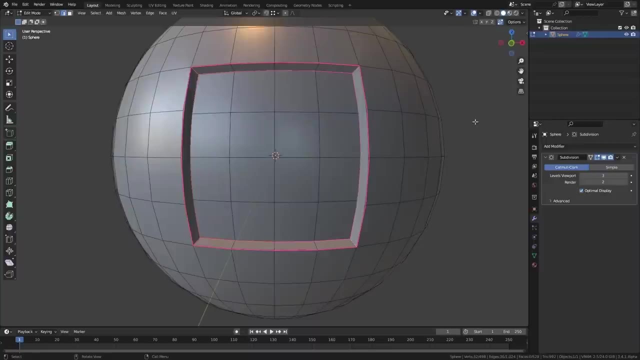 lines go pink And if we enable the subsurface again we can see we've got these nice hard lines and we don't have any of the weird pinching or issues that we had before. And the best thing about crease is you can always go back and press, shift and E again and you can reduce. 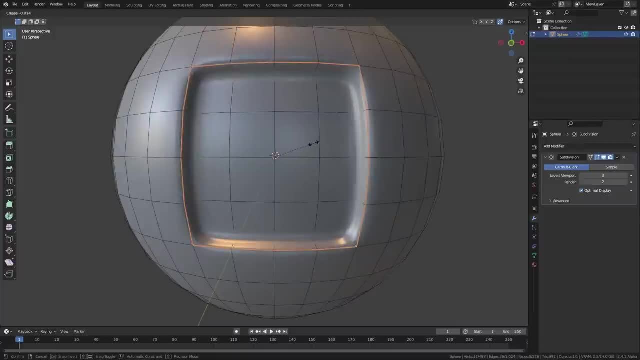 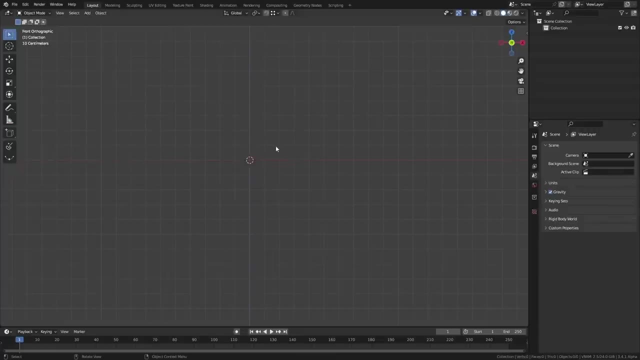 the amount of crease, So you get exact control over the whole thing. So that's all well and good if you're wanting to just extrude in and out of faces that already exist. But what if you wanted to say, boolean, cut on a curved surface? Well, that gives. 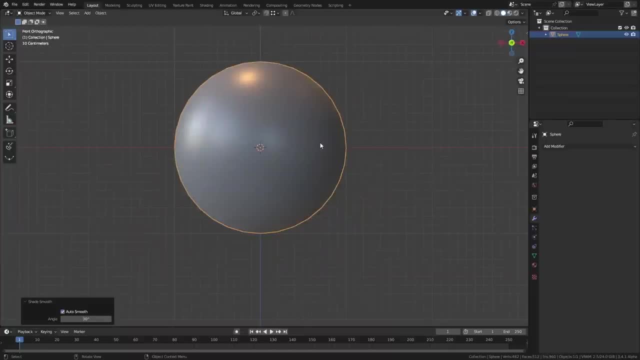 us some new problems. Let's just add a sphere here and shade it smooth. And then let's say we're going to cut out a cylinder, which is quite a common thing to do. What a lot of people will do is they'll think, oh well, I want a nice smooth cut. So they'll really 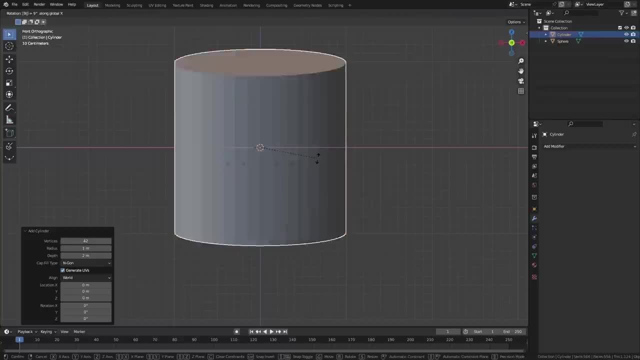 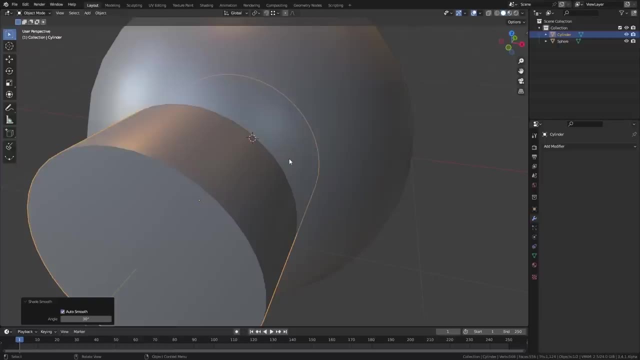 ramp up these numbers to something like 42.. And they do, And then we'll rotate this. I have the bool tool enabled, which is just an add-on that comes with Blender, And it makes it easier to boolean things with just a shortcut. So 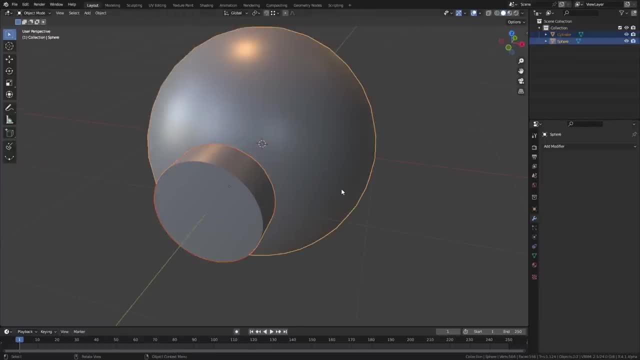 I'm going to select both of these And I am going to press control and minus And that'll cut that out And you can see the problems that we're getting here. We get these weird glitches right And if I make this smaller, the glitches will probably get even worse. 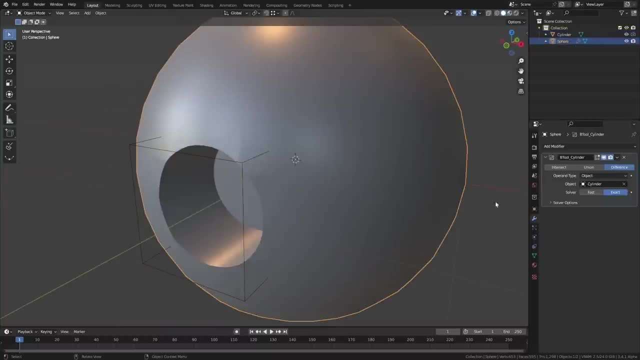 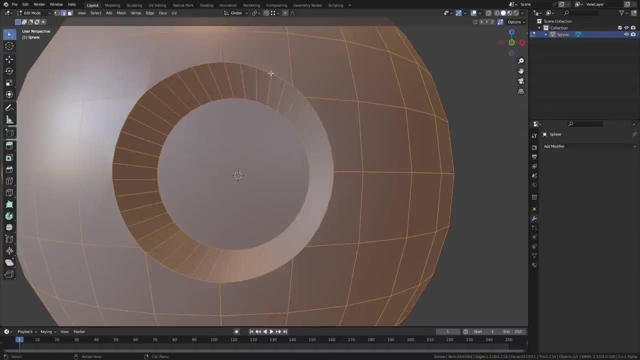 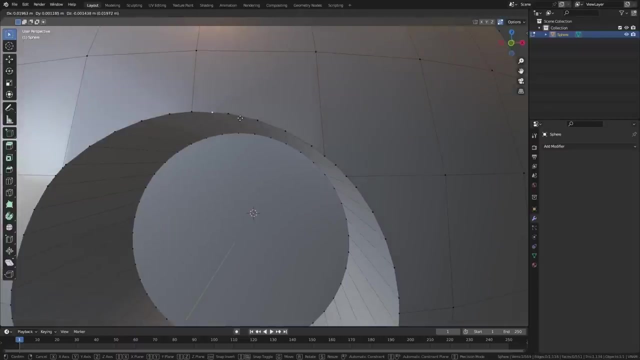 Yeah, So the reason why we're getting these glitches- if I apply this, we'll see, Because I used a very dense mesh there. Especially, We have all of these new edges that have been added, But each one of these verts, that's what's causing the problems. A face has to be flat, And when you're cutting, 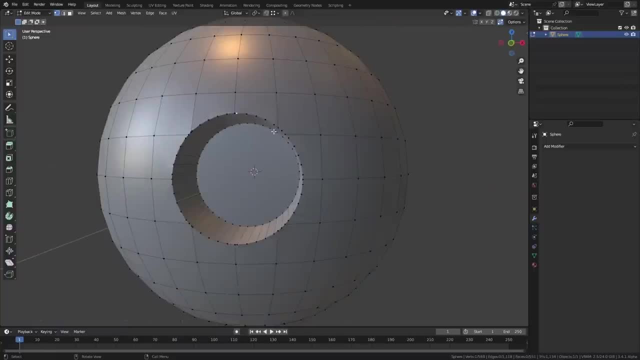 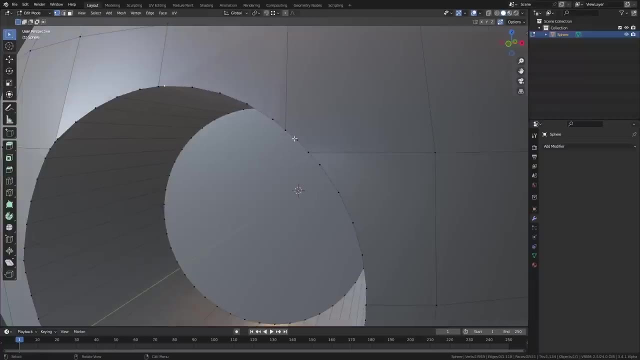 out a shape on a curved surface. you're now making these faces not flat anymore. We can fix this quite easily If we go to options and auto merge. what we can do is just find all of the near misses, And we can double tap G and just slide them into the nearest. 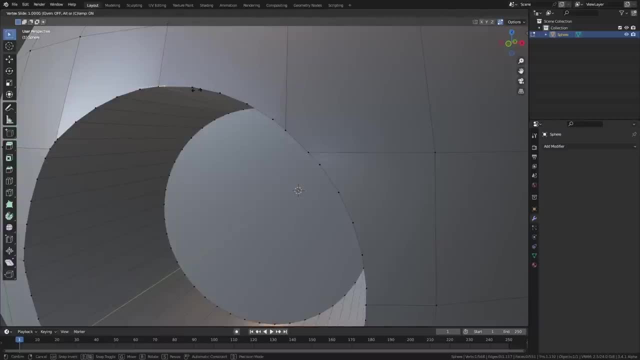 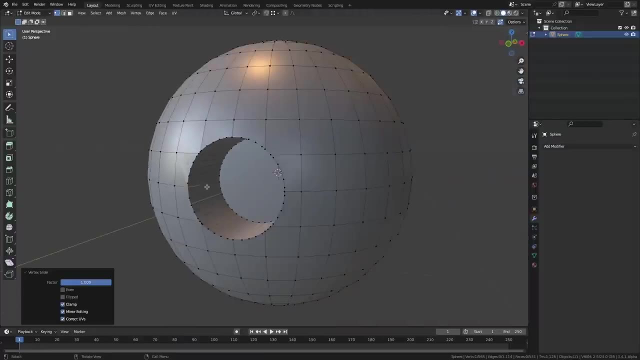 neighbor And you can see there how that fixes this problem. And if we just go around most of the near misses, that should fix most of the issues. Now, the reason I think density is so important for this is because if we used a cylinder, 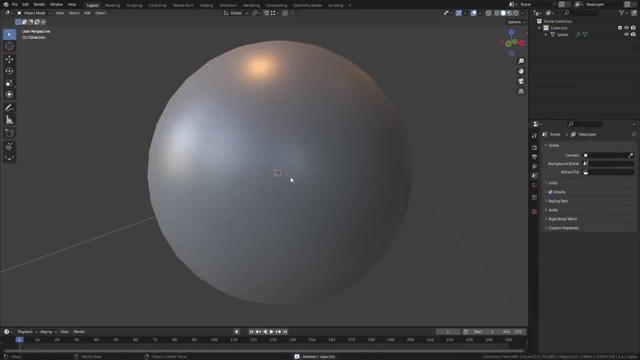 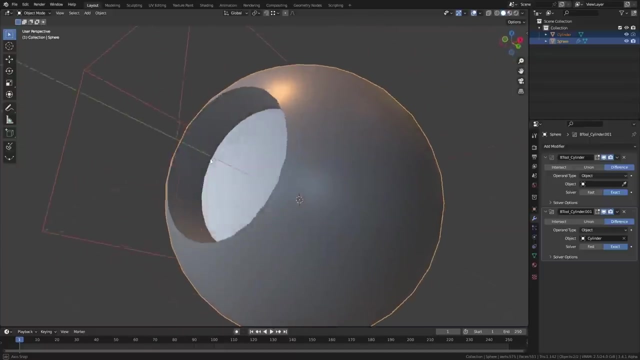 that didn't have as many edges, right? If we used a cylinder that was, let's say, 24, and we do the same thing now. we have a lot less to clean up. In fact, this is that's clean, right off. 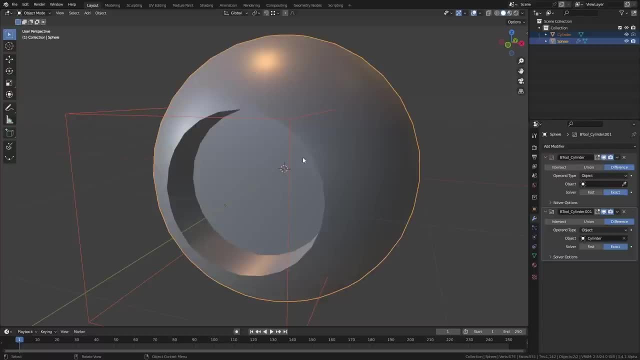 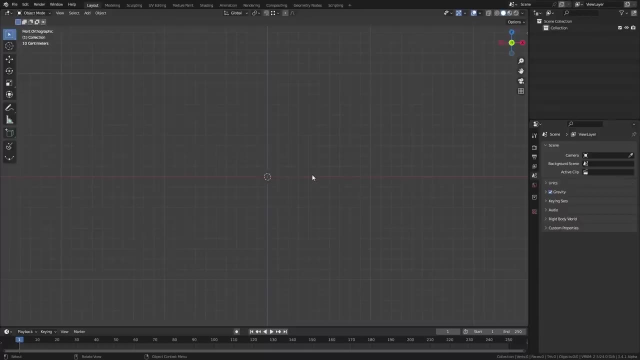 It's a lot easier to balance. pretty much There's one or two errors that would have to go in and fix, but it's much less work and it's a lot. it's going to give you much nicer results. The next tip that I want to talk about is making T joints. It's really common in a lot. 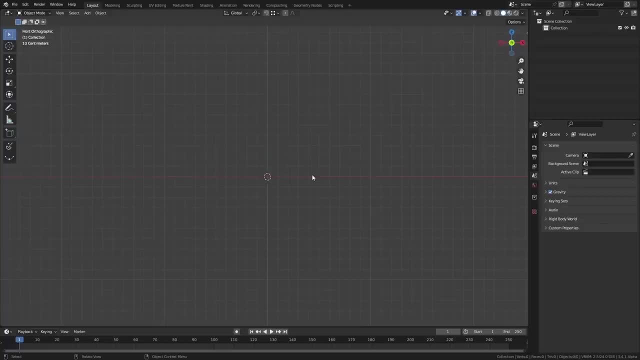 of objects to have two metal cylinders or something like that on, say, a railing or a handle, where you'll have a 90 degree connection between two different curved objects. So let's just add a cylinder into the scene again. Yeah, just like that. And then we're going. 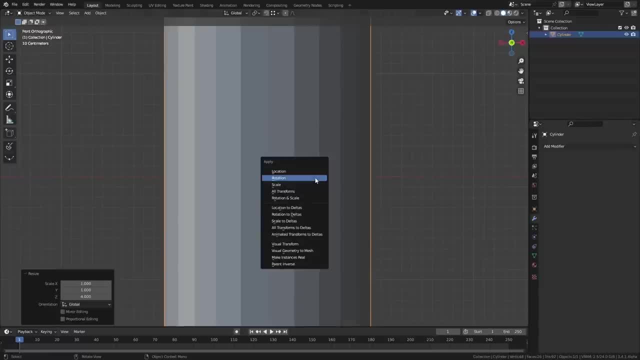 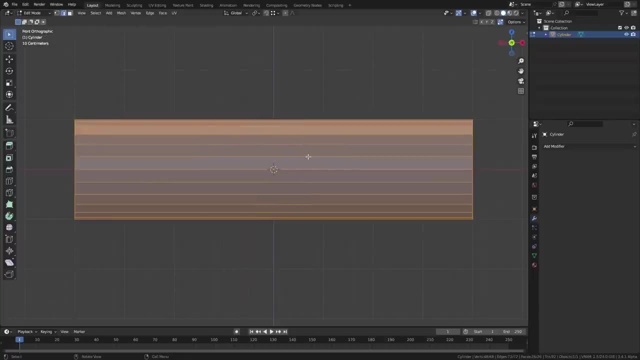 to do the same thing. Yeah, 24 should be fine, And I'm going to make this about four times longer and apply the scale And then the first method that everybody learns, the thing that most people do is they'll just use the knife tool, right, Add an edge in the middle here and we'll. 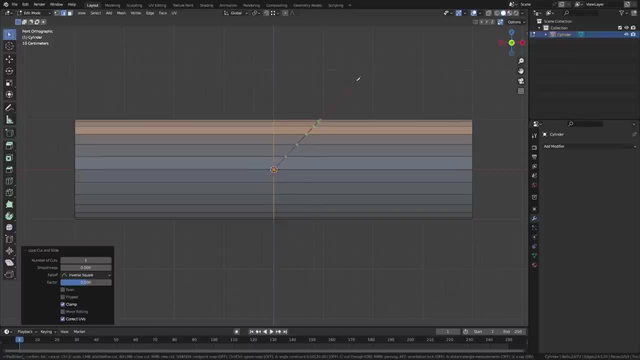 press K for the knife tool And then, if you press C, it'll cut all the way through the mesh and you can press A 45 to cut at a 45 degree angle, Right. So let's just mirror this so we don't have 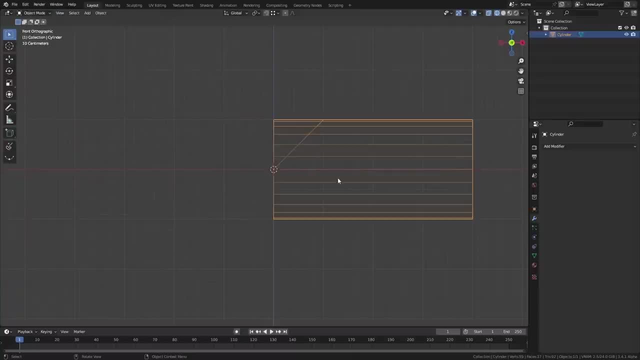 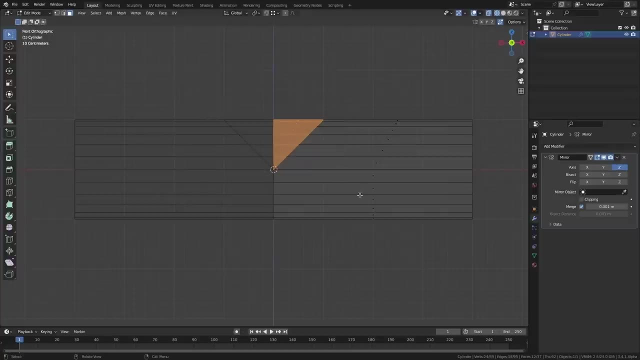 to do everything twice. So let's just mirror this so we don't have to do everything twice. I have mirror set up as a shortcut here, So then you can just select all of these faces that we just made and you can extrude them up, And now we have a cylinder. But sometimes 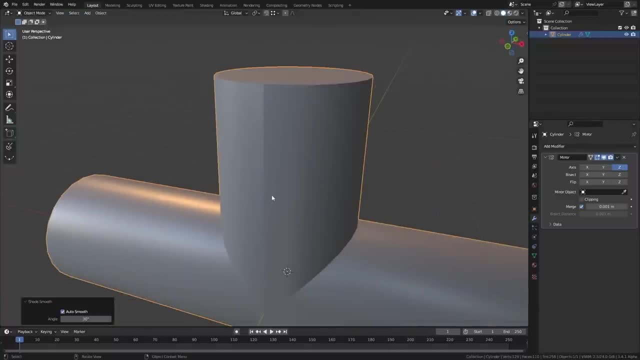 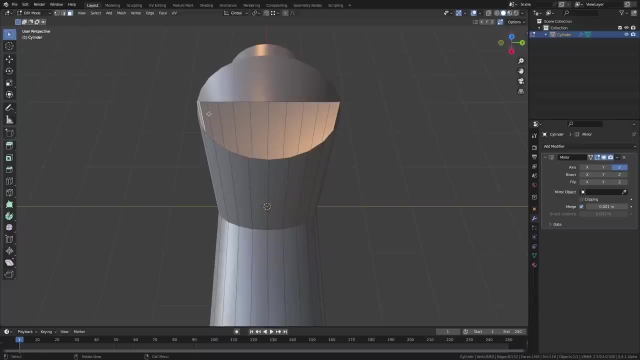 this causes really weird shading glitches like this where you have this line down the middle. You also have to go through and you have to delete these faces. And then you have to go through and you have to delete these faces, And there's a lot of cleanup work to 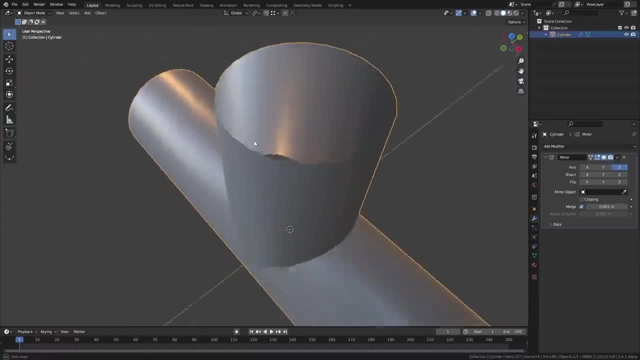 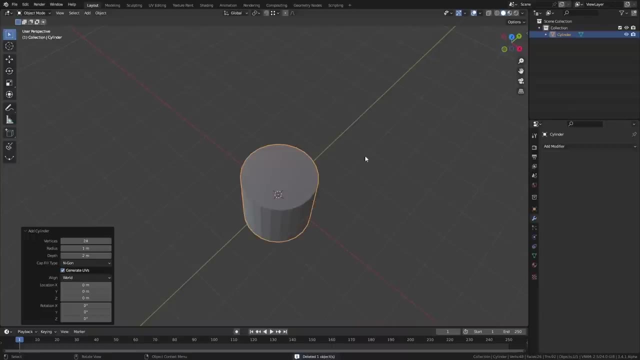 do, But ultimately you still have to end up with this weird kind of glitchy looking thing. so we can- we can do this better, basically, and the way that I prefer to do this is to just grab a cylinder. I'll make this for game, and we can actually just use a boolean cut if I. 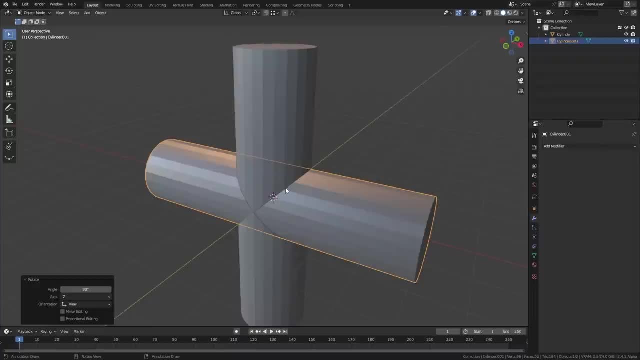 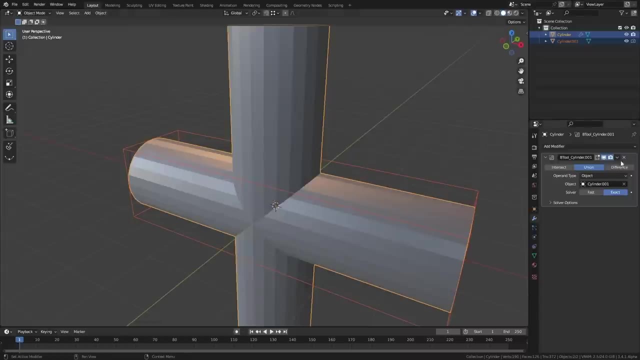 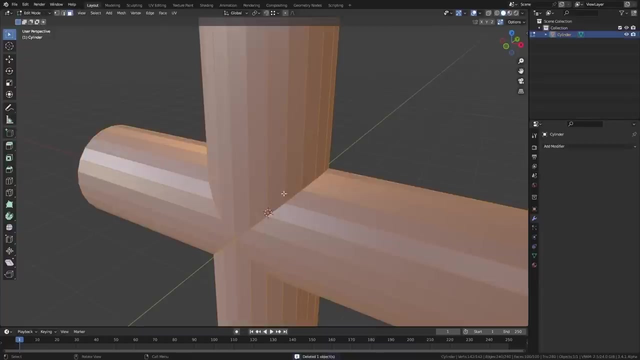 duplicate this. I rotate around to make a t-joint and I select both of them and I press ctrl and add. the bull cutter tool will add these two together and because they're the same size, you actually get really nice topology and then I can just apply that and get rid of the joining object and you can see that we've got. 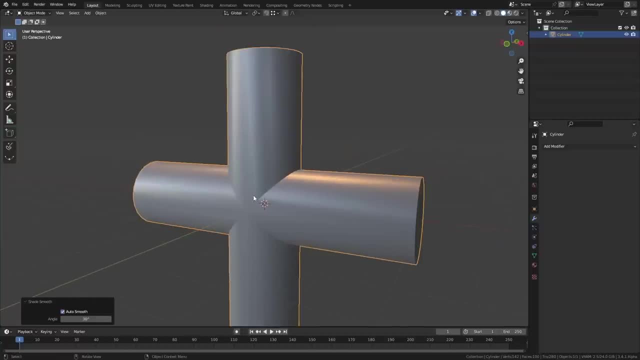 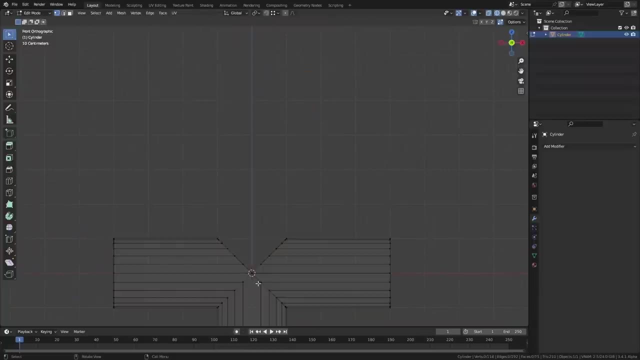 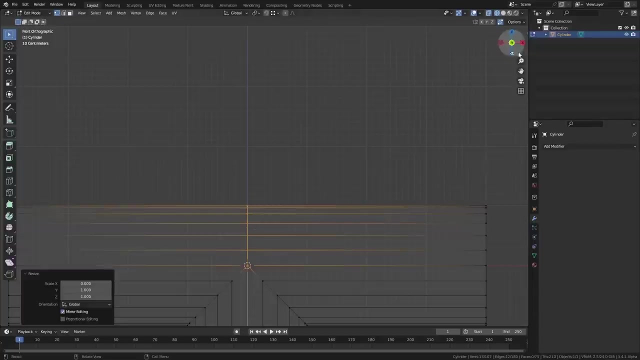 pretty good topology and if we shade this we don't get the weird line. and if we want to make it just a single joint, like we had last time, we just need to get rid of these verts, select these ones and press scale X zero. and because I've 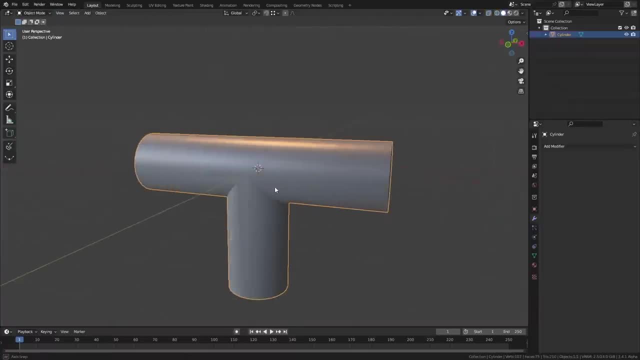 got auto-merge on, these will merge together straight away and now we have a really nice topology and you can see that we've got a nice topology and we really nice looking joint and then what we can also do is just grab these edges. here we can bevel. 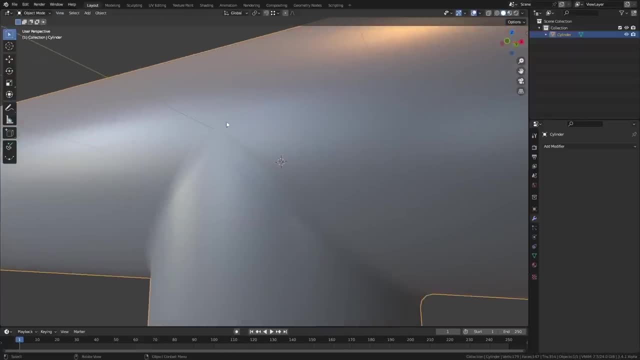 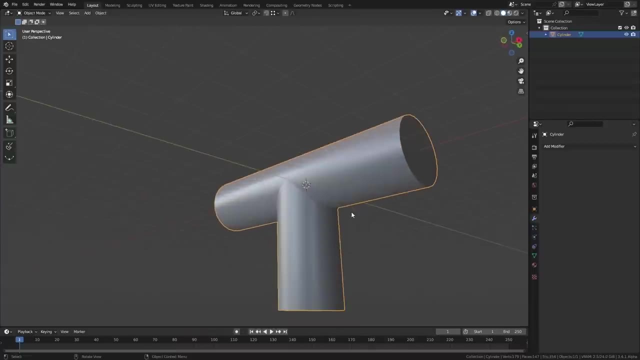 them a little bit, we can get a nice smooth, kind of like a weld look like two pieces have been welded together. so I think that's a much better way to make these sorts of joints. I think this is a really important tool to have in your belt if you're doing a lot of 3d modeling, because this 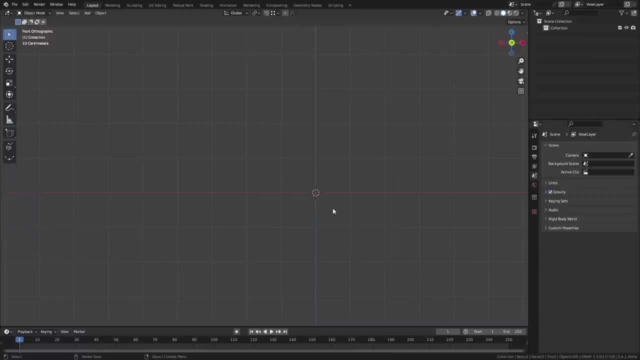 shape appears all the time. okay, so next up, let's talk about radial topology. a lot of times when people try to model something radially, it's really off-putting, because you have to either do the same thing over and over again, or you model one small section of of the object and then you rotate it. 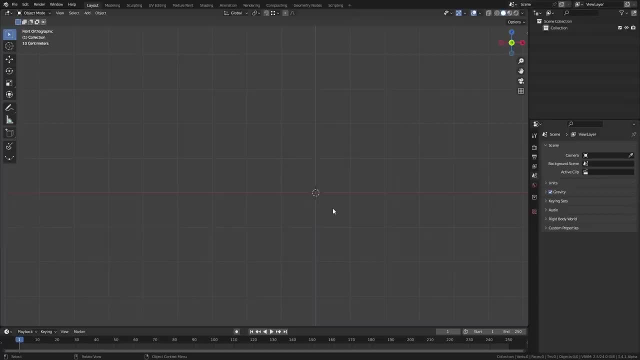 around and duplicate it, but that's kind of awkward because then you have to know the exact scale that you want to model to, or people will use a boolean and that causes all sorts of problems with topology. so what I prefer to do to keep the topology really nice is: I'll just add in a plane: 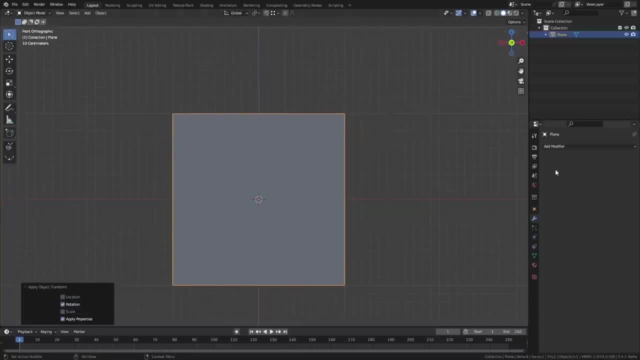 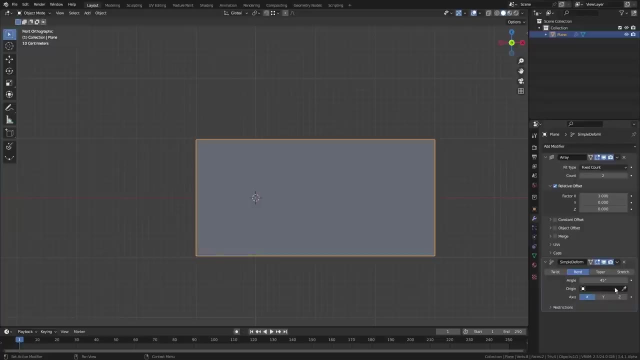 rotate it 90 degrees, apply the rotation. then I'll add an array modifier and I will add a simple deform. we set that to bend at 360 degrees on the z. what that'll do if we up the count on the array? it'll just keep continuing. 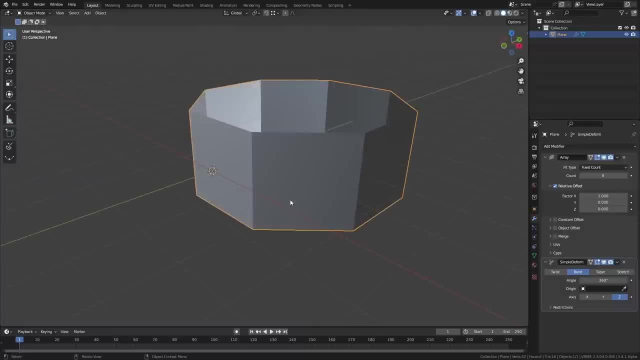 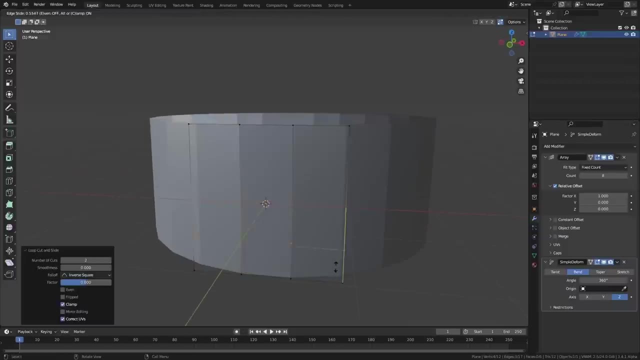 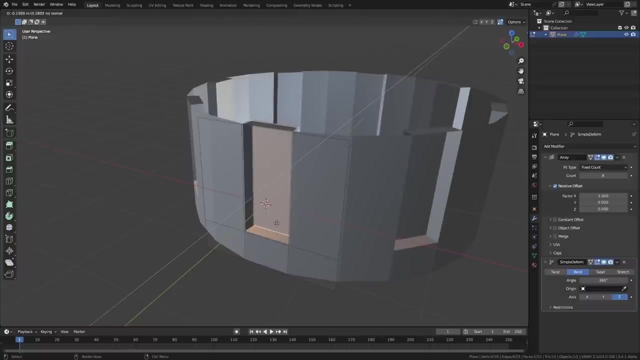 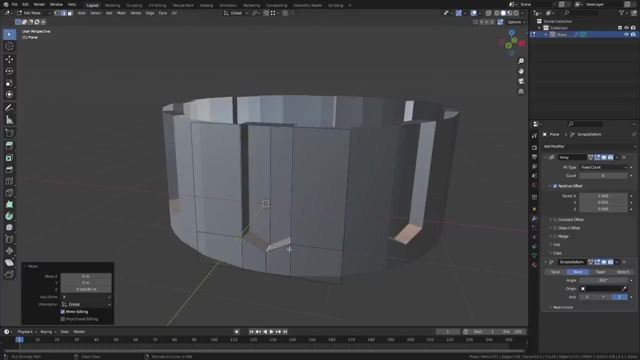 the same thing around again, again, again. so now, if we went in and we tried to do something like, I don't know, like a revolver right on a revolver, you get this kind of design way. you have something like this- maybe this would come down a bit, bevel that- and you get something like this on the chamber of a revolver. 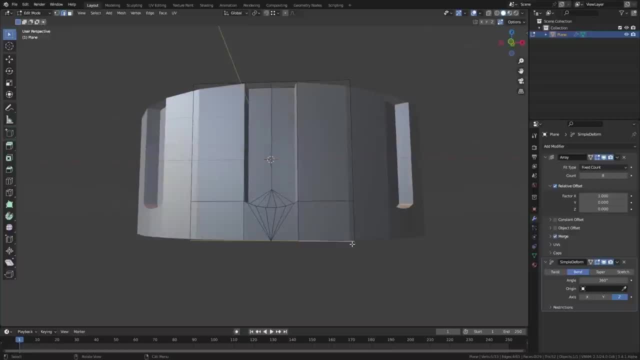 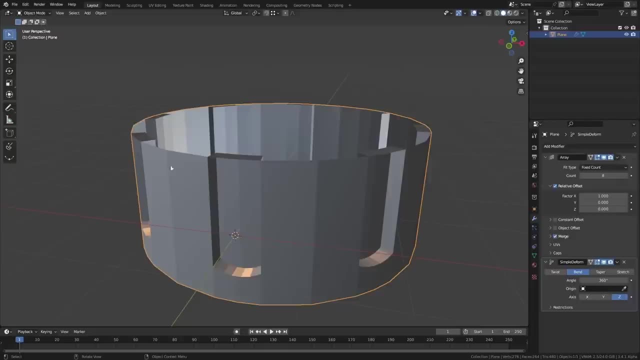 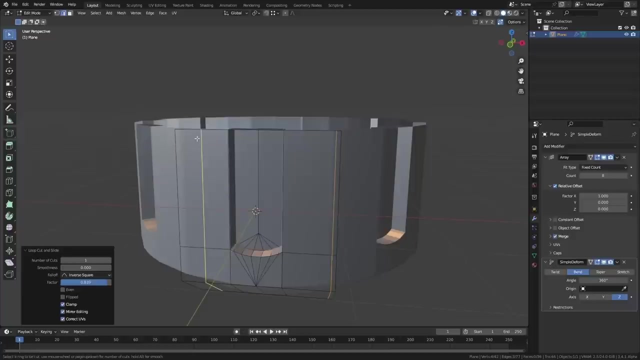 we can press merge as well, to merge all of the array together, extrude that down and then move that in, and you can see that we have these very visible seams in between. and that's really easy to fix as well. all you have to do is just move a. 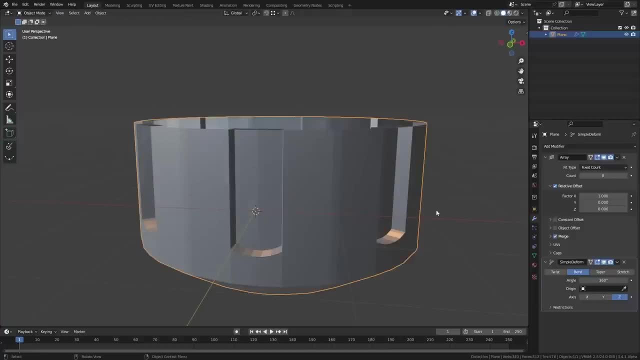 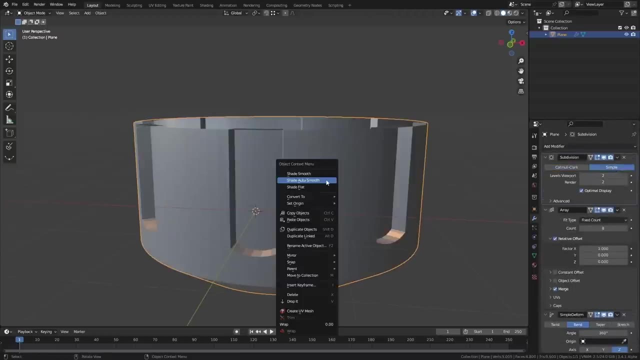 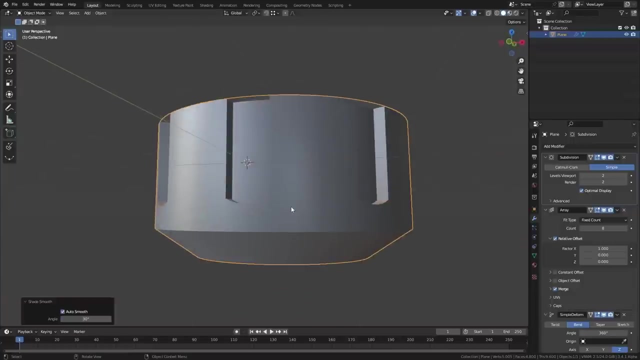 supporting edge near there, or a few supporting edges, and you can also add a subdivision surface modifier and move this to the top. change that to simple. let me shade, smooth this and we get this really nice topology. it's all quads and you can just keep modeling on on a radial manner, which 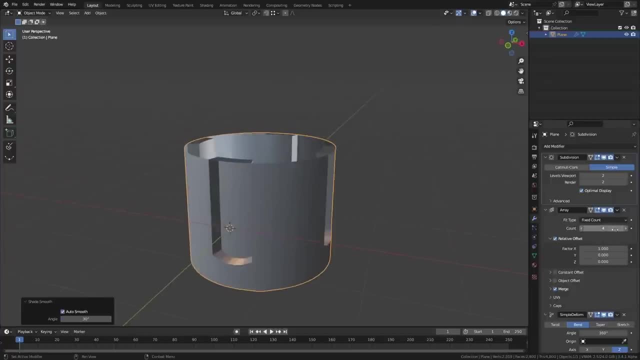 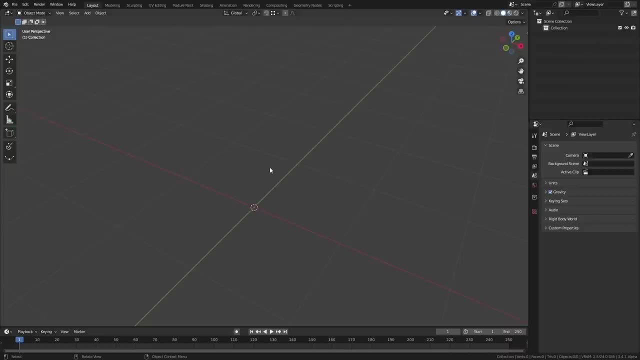 is basically procedural, and the best thing about it is you can always just change the model count as well, which is something you can't really do if you're modeling any other way like this. the final tip that I want to talk about today is about cylinders. cylinders are quite 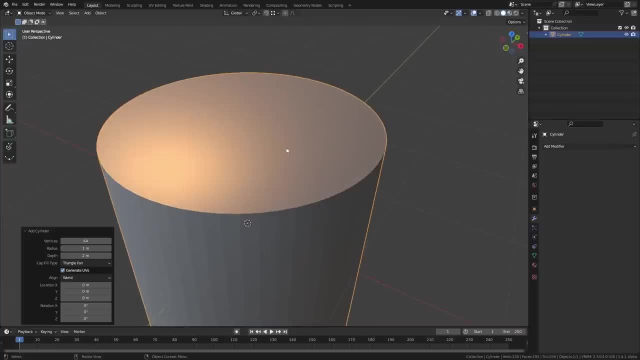 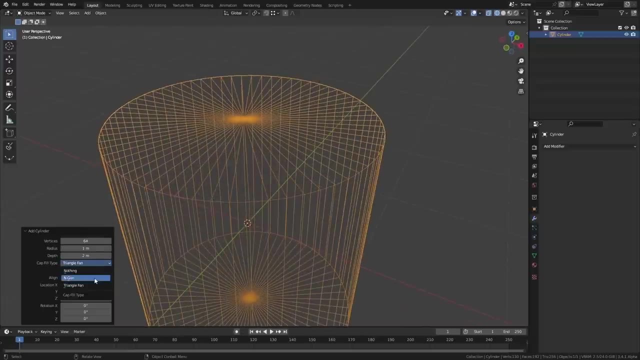 hard to work with with nice topology sometimes, because when you generate a cylinder, among other things, the top is either a triangle fan, which is a load of tries going into the middle like this, or it's one big and gone. and the problem is if we add a subdivision surface modifier to this.